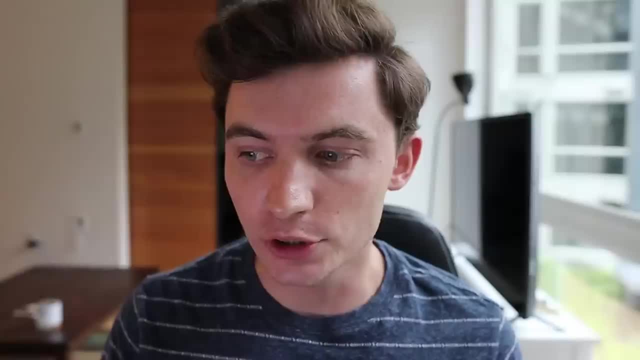 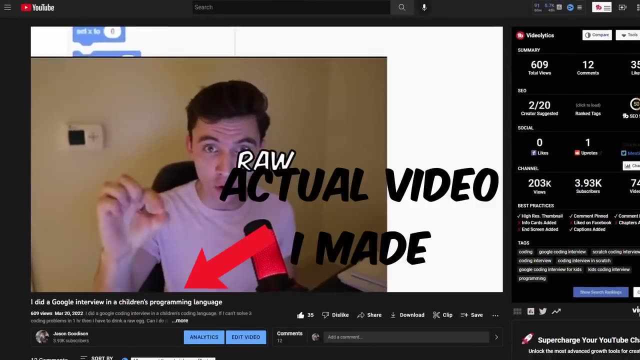 to tell you what I did. I started coding in grade 11.. Well, sorta, We started with this language called Scratch. It's basic game development made for children. Nobody would be stupid enough to, let's say, do an entire Google coding interview in this language and 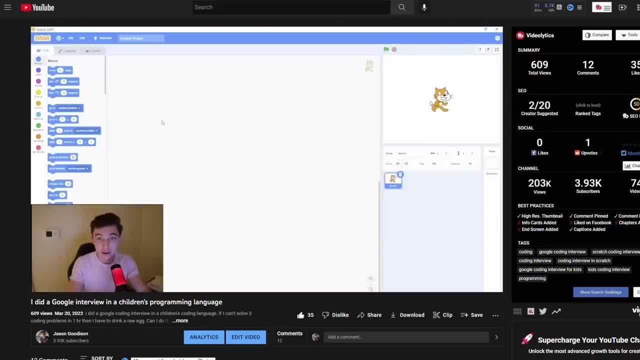 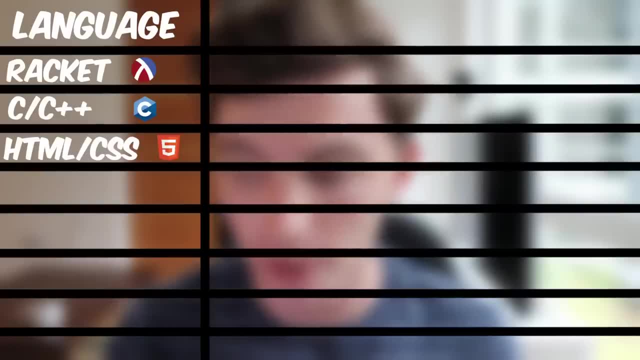 maybe even do shots every time the code fails. So let's just skip that and get to the important stuff. I went to Waterloo and, in order, I learned first Racket, then C, C++, HTML, CSS, TCL, Python, Java, JavaScript, C Sharp. Some of these were in class, some were on their own. 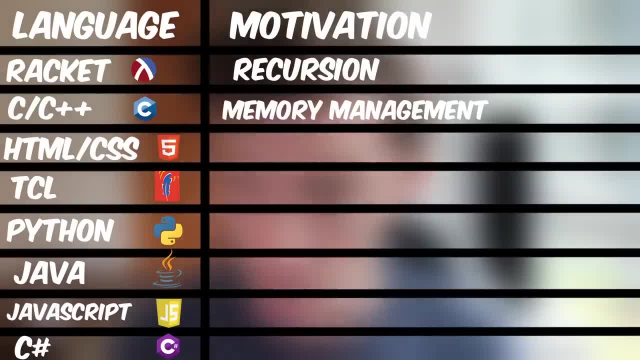 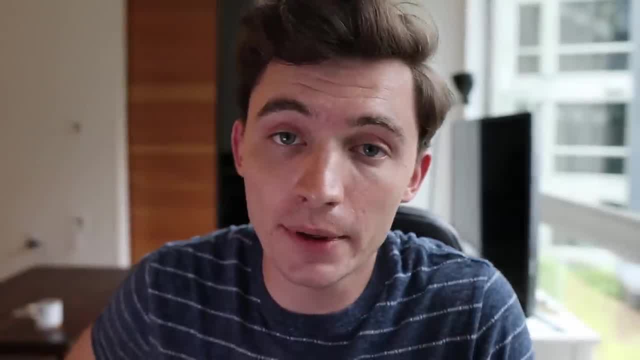 Here's the motivation behind each Racket for recursion, C for memory management, C++ for object-oriented design, HTML and CSS for web development. although these are not real programming languages, they're markup languages. TCL- I did it at an internship and it's fucking. 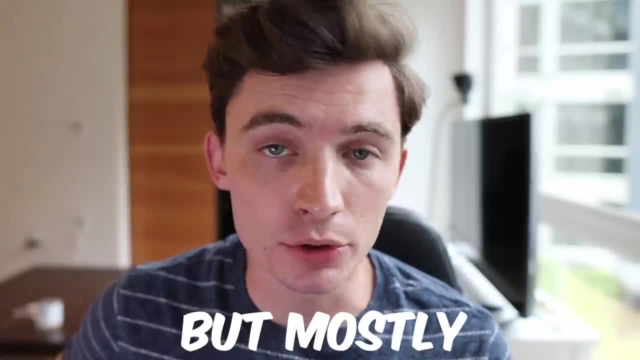 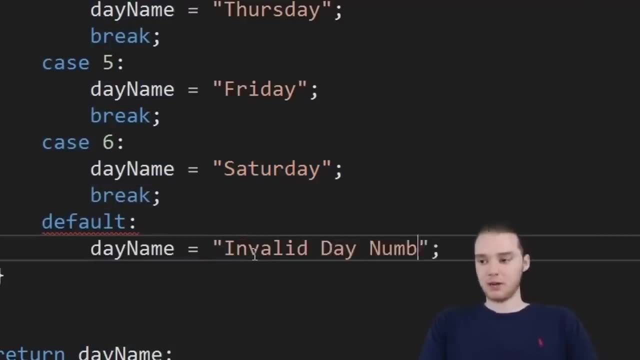 useless Python. I learned this alone and over time, But mostly just for side projects. Java and JavaScript for back-end and front-end web development And finally C Sharp, which I do for my full-time job now, but it's essentially. 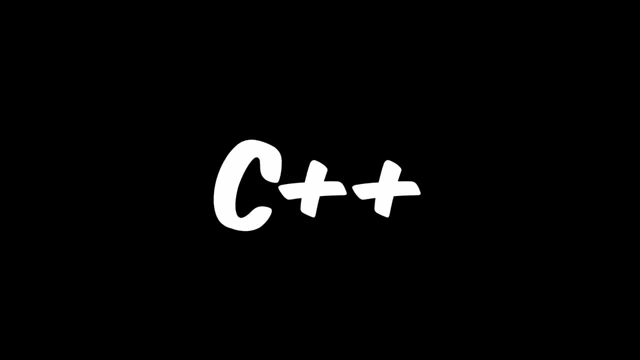 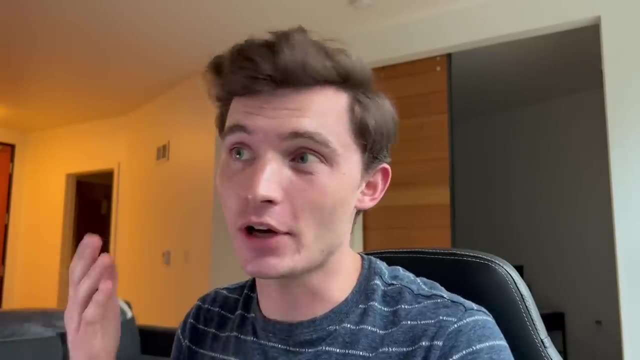 Microsoft's version of Java, so let's not talk about it. C and C++ are by far the most useful languages to learn. After I learned those I realized most other programming languages are essentially just derivatives of those. Each new programming language essentially takes those and makes some specific task easier. Basically, all. 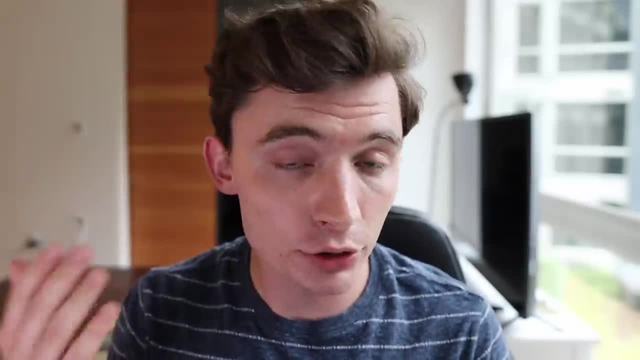 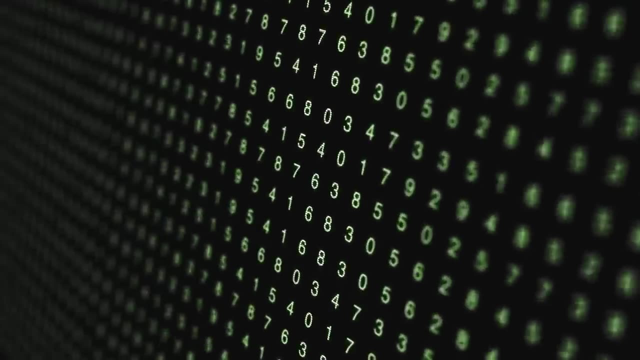 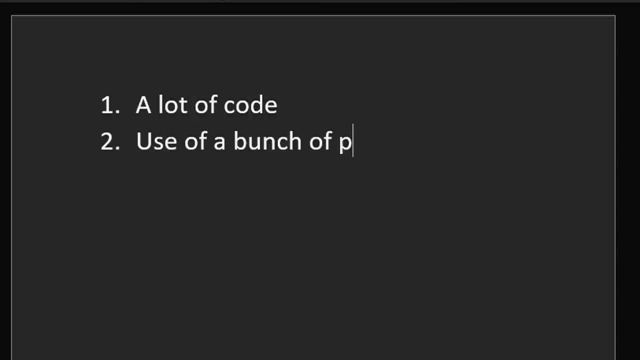 these languages share the same ancestor in C and C++, So clearly you should start by learning these two languages, Right? No, These languages are pretty intensive. If you want to do anything useful or impactful, it either requires one, a lot of code, or two use of a bunch of libraries that you've never. 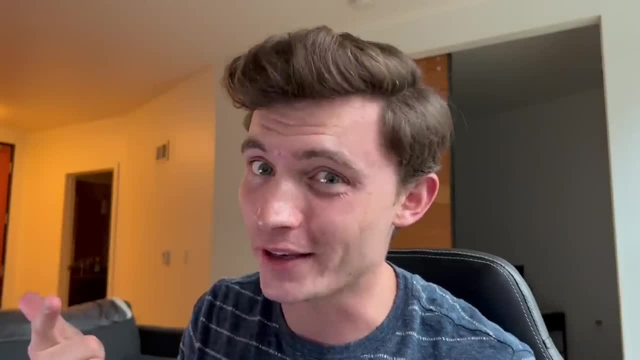 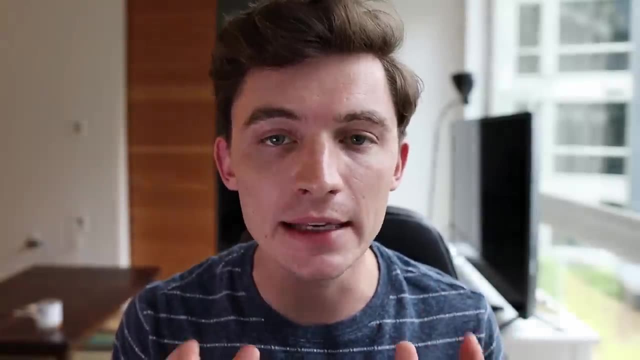 heard of before and, honestly, are probably not worth learning. Which brings me to my point. You need to do something useful, but not too useful. Now hear me out. If you're learning C, it's going to be relatively easy to start solving some. 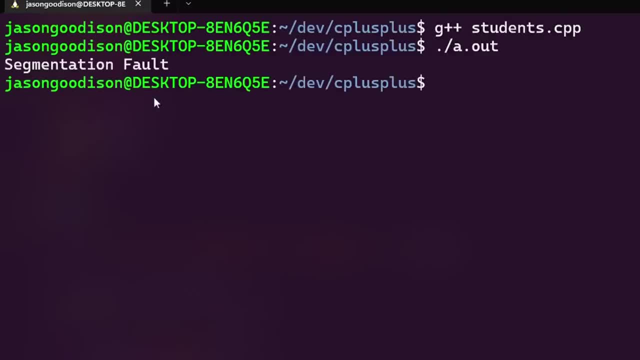 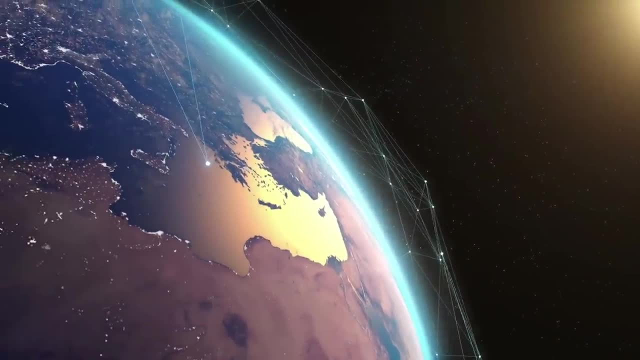 basic math problem and you'll print the solution on the screen. But all of your code is contained into this, This little terminal. If you want to make a graphical game or connect to a website or do anything, quote unquote useful. it'll actually be really hard, Like even for me right now. 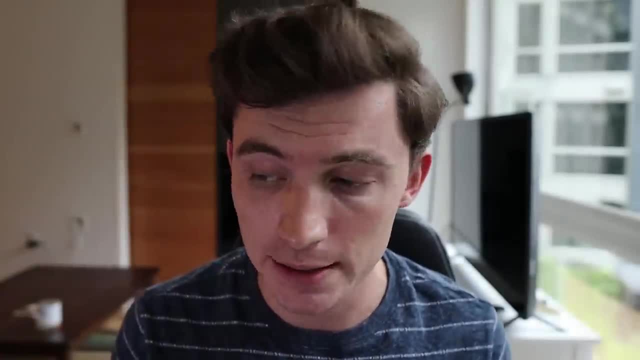 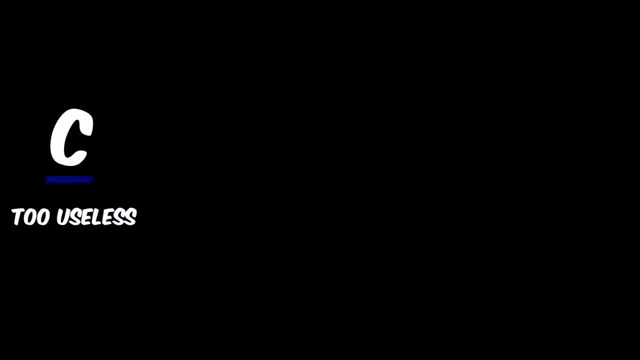 I would have to do a lot of Googling to even figure out how to do those things. Essentially, if you start with C, anything useful is going to be too hard and this will be really demotivating. Now let's look at the opposite end of the spectrum. Many students want to get into coding. 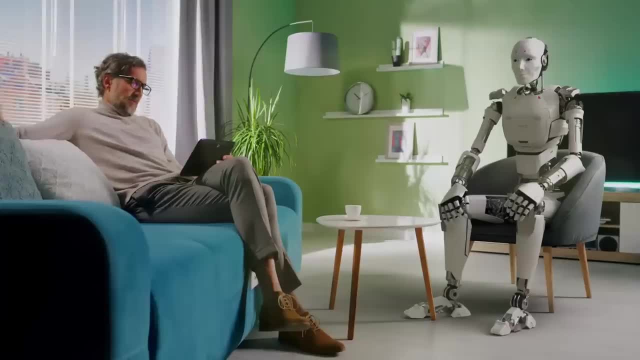 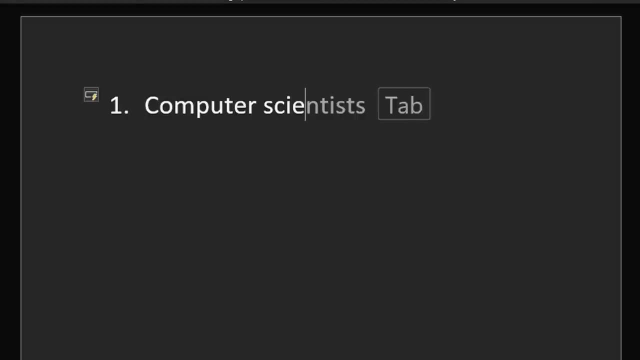 and the first thing they want to do is learn machine learning. Here's the thing: Machine learning is super useful in the real world, But Advanced math. So if you start with it, you're going to be learning one: computer science basics. two. 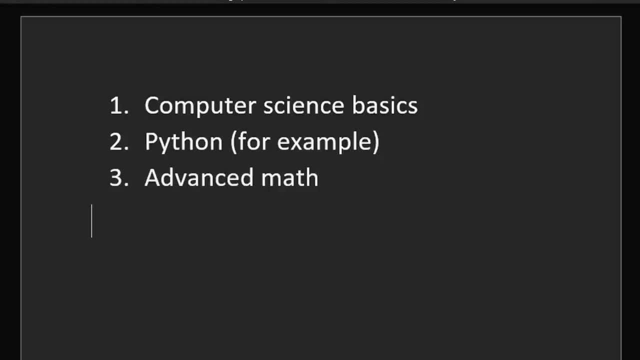 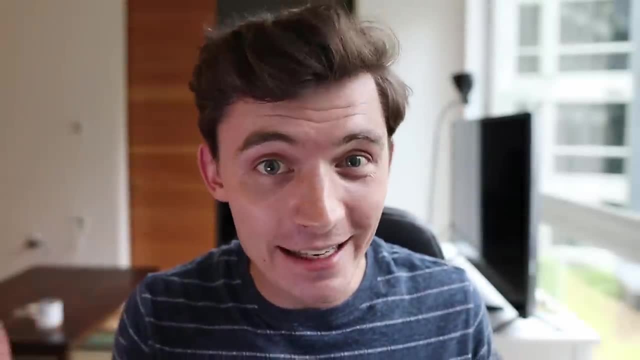 Python, for example, and three advanced math topics all at the same time, And unless you are literally a f***ing genie, you're going to come out of that not really knowing any of the three. The sweet spot is somewhere in the middle. You need to do something. that's useful, but 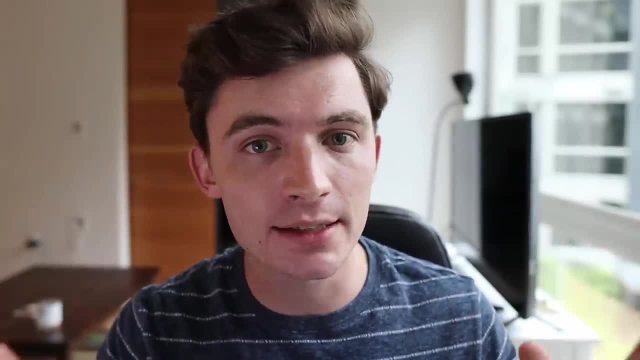 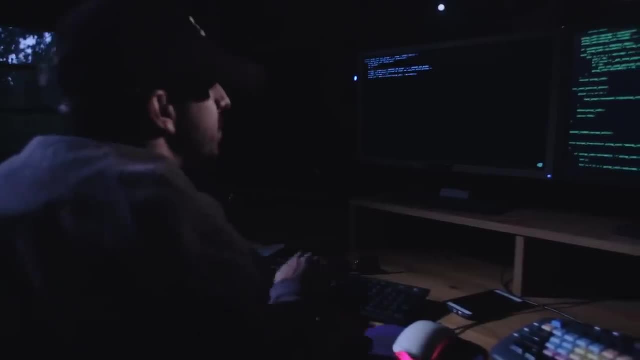 not too useful. Now that we're talking about doing useful things, let's clear up the distinction between coding and programming. Coding is just writing code to solve computer science problems. Let's call them math problems to show the distinction. This is what you need as a prerequisite to 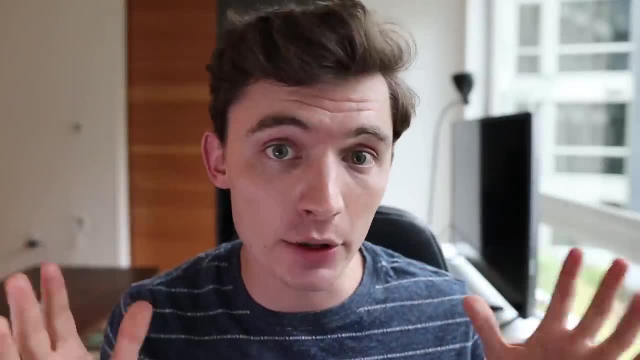 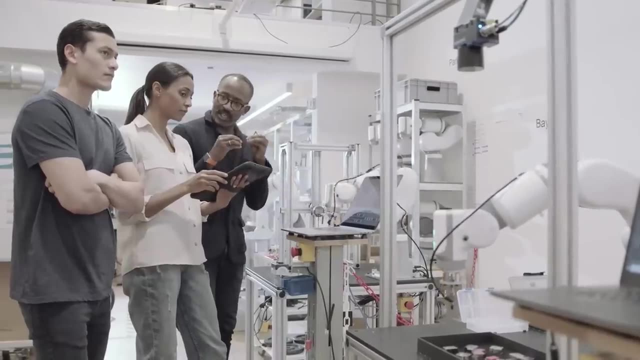 learn how to program. Programming is the ultimate goal. Programming is the act of using coding to make programs that solve real problems. You need to learn the fundamentals of coding to know how to program. Remember when I talked about people starting at machine learning. 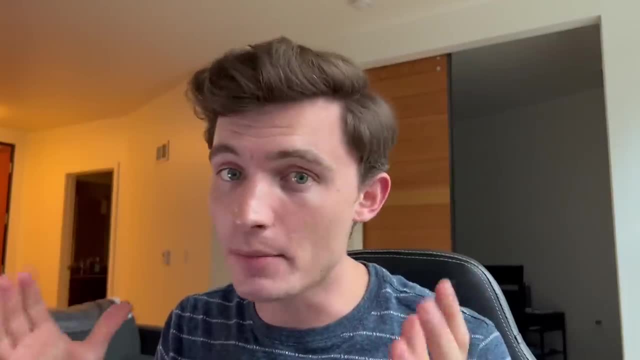 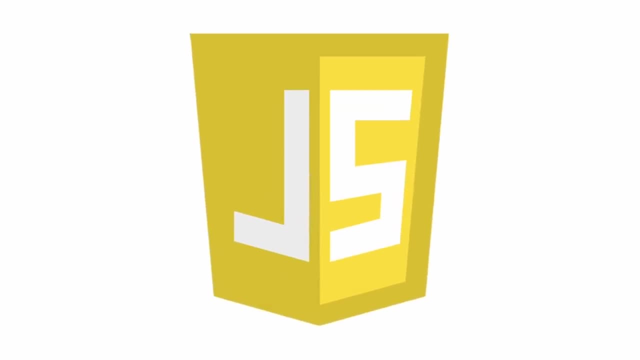 the basics of coding. You need to learn the frameworks that surround each coding language, But in the beginning you kind of need to isolate the coding language itself, learn the basics of that and then you can take it and learn how to program with it- The easiest thing. 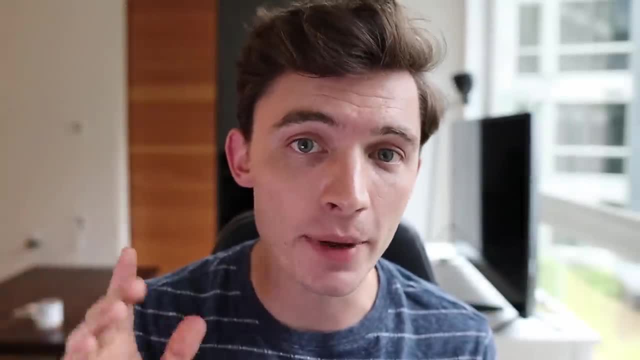 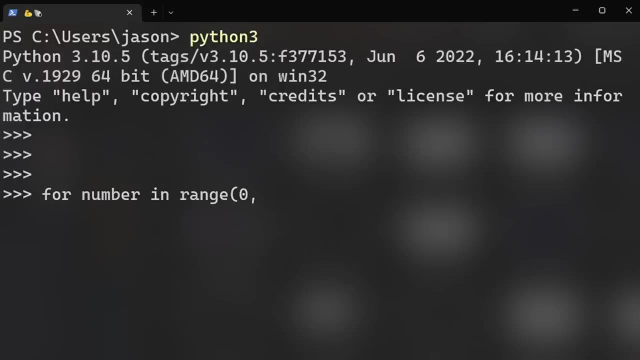 to start with is probably Python, But honestly I wouldn't be upset if you picked a JavaScript and I'll explain later. Python mostly looks like plain English. Even if you don't know how to code, you can sort of read it. It's super easy to get started in. You can immediately start learning the 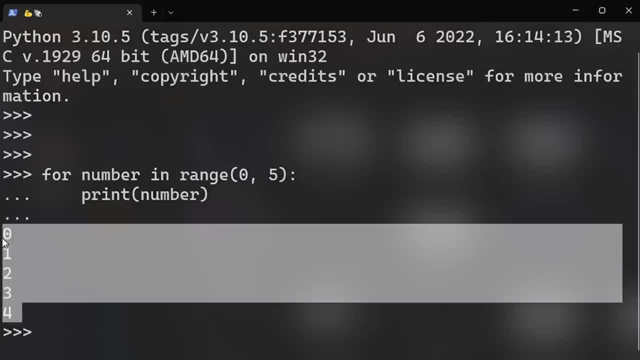 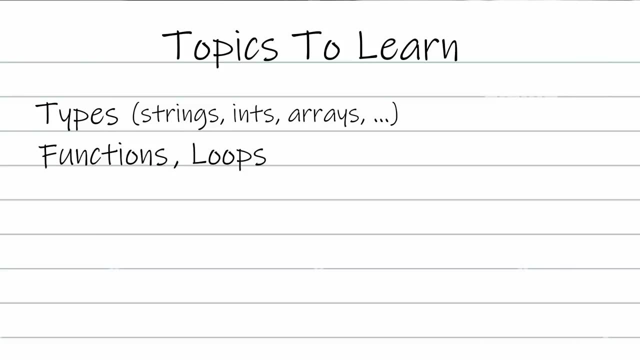 basics, like variables, functions, move quickly into data structures and algorithms. You'll really want to know the basics about types, like arrays, and the basics of control flow, like functions, loops, and even a little bit about classes. Don't get carried away, You. 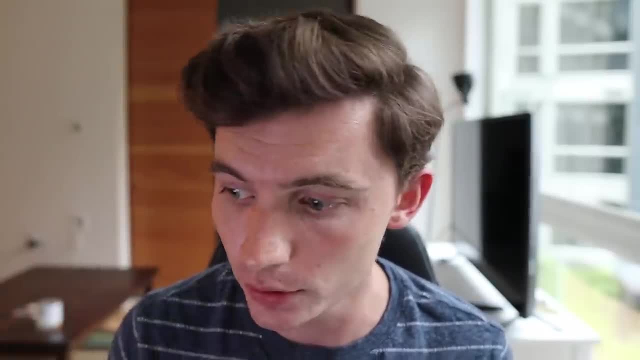 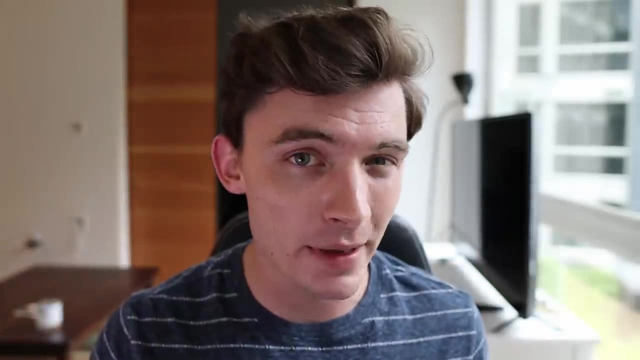 don't need to learn advanced things like inheritance, for example. If you're feeling a little feisty, you might want to learn exceptions, hash maps, maybe sprinkle in a little recursion. Now there are plenty of intro to Python courses in the world, so I'm not going to bore you. 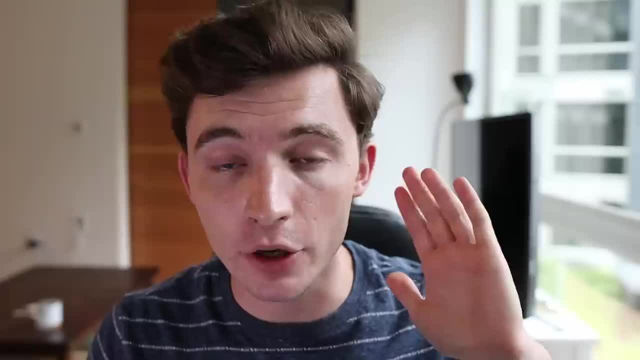 with the details. I'm sure you can find that on your own. But now that you have a coding language down, let's talk about programming. So the first thing I would do is I would start with programming. So the first thing I would 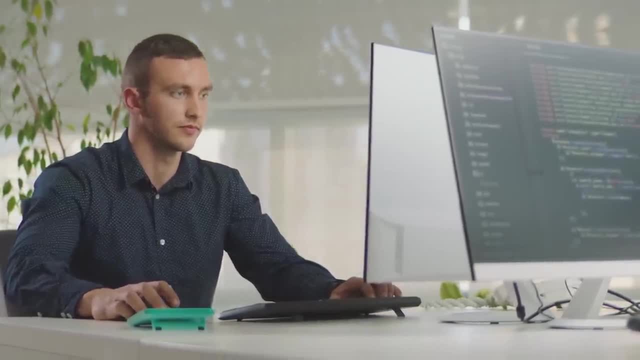 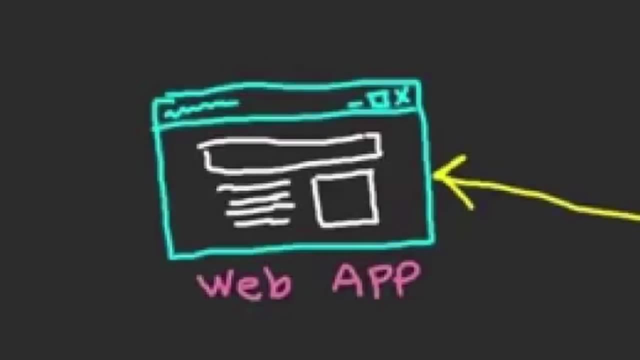 do is take what I've learned and build a website. Now there are three important aspects to a website. There's the back end, which kind of manages user data. There's the front end, which is what runs on the user's browser, And then there's the database, which essentially 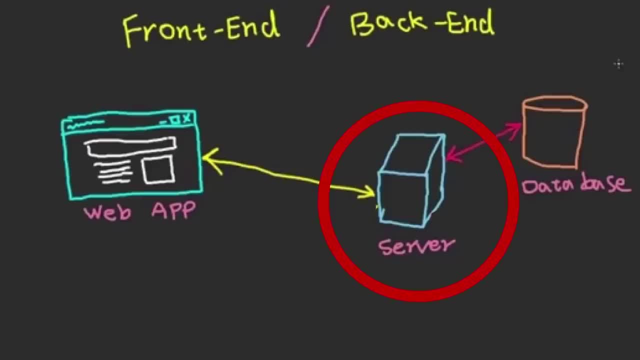 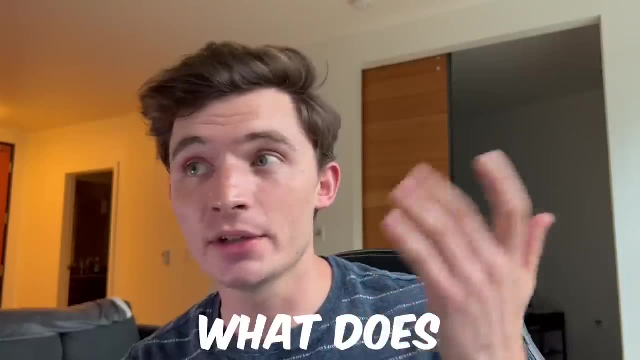 just stores data. Now we'll start with backend. You're going to want to pick a pretty high level language, either one Python or two JavaScript. The first program I would build would be a basic website. Now, what type of website? What does that website do? Well, I'll explain. 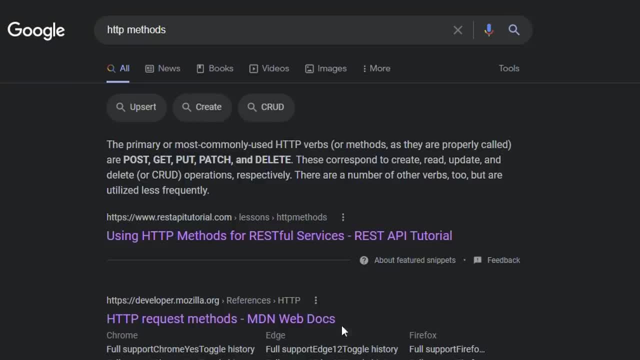 that in a minute, But for now, let's just make a project in that language. Now, when making a backend, you're going to learn concepts Like HTTP methods, GET, POST, for example. Depending on the project, you might be interacting. 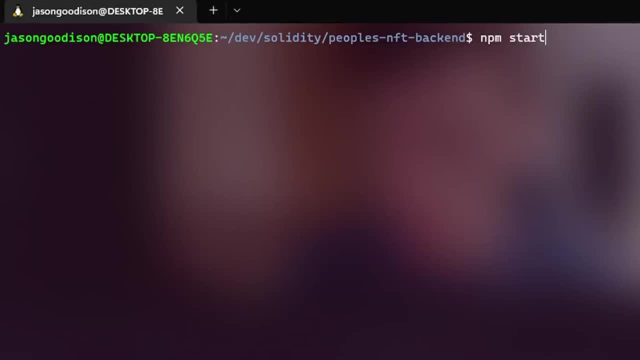 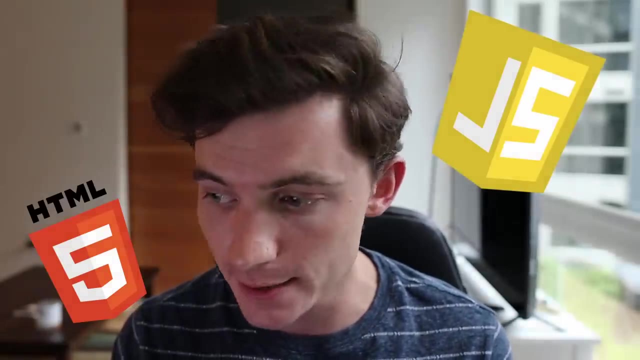 with a database. Once you start to feel comfortable and have your basic backend working, then let's try our hand at the front end. Now, on the front end, you're going to be using things like JavaScript, HTML CSS. This is the reason I said JavaScript is actually a pretty good. 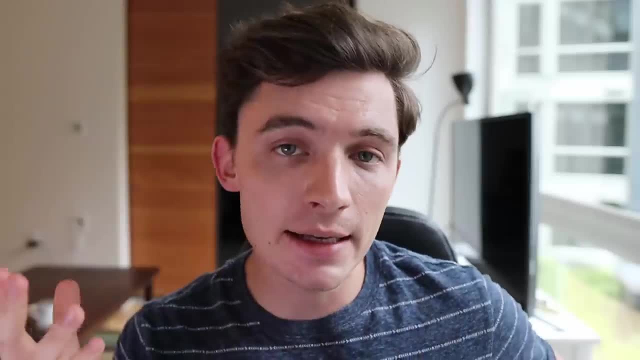 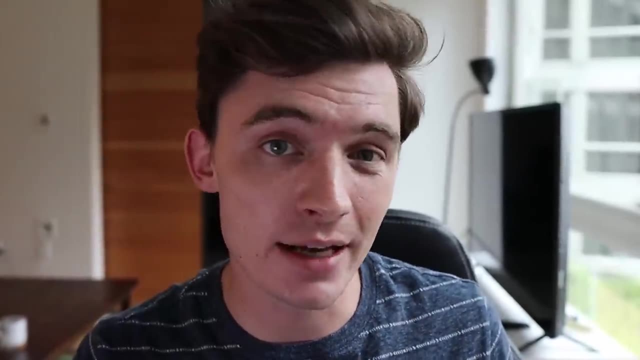 starting language, because you can use it for the backend and the front end. Now I said, each programming language has a bunch of tools and frameworks that make it easier to use. Basically, there's no reason for you to write code that somebody else has already written. 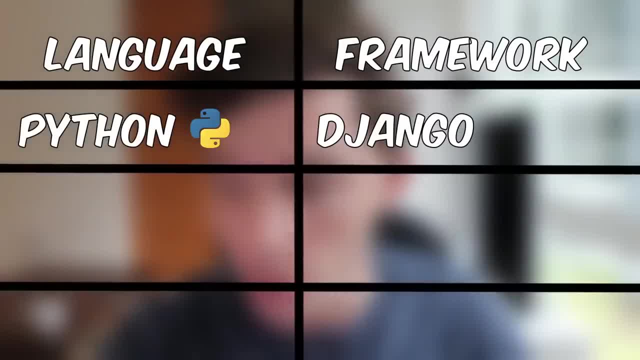 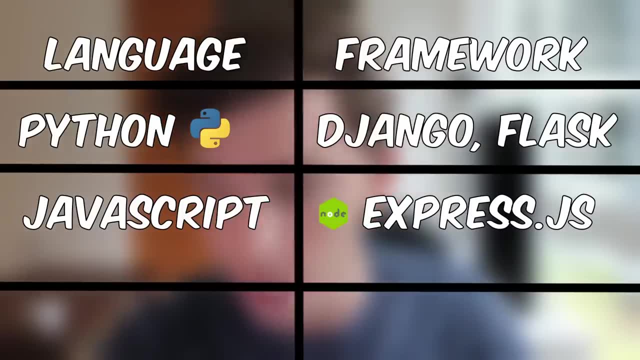 The frameworks I would use for these languages would be Python. I would try either Django or Flask JavaScript. on the backend, I would use ExpressJS, which just think of it as simplified Nodejs, And on the front end I would use React. And if you need a database, I would. 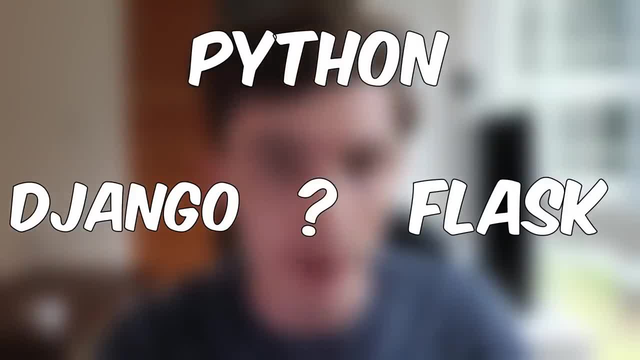 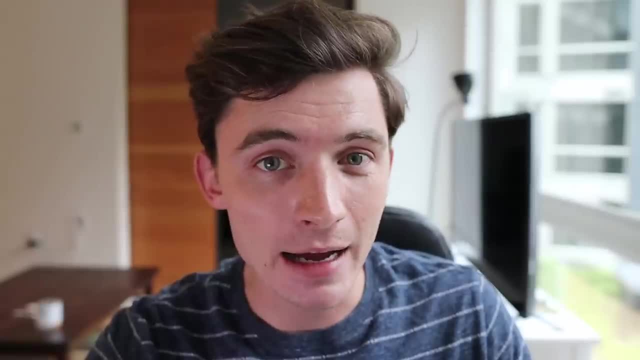 try MongoDB Now. anecdotally, I can tell you for Python I've seen more jobs listed for Django than for Flask, And I've seen more ExpressJS jobs over Django On the front end. I think React is pretty solid. After that time you should learn C and C++ as it'll. 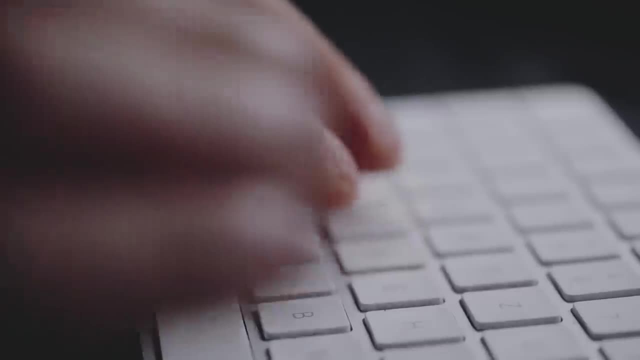 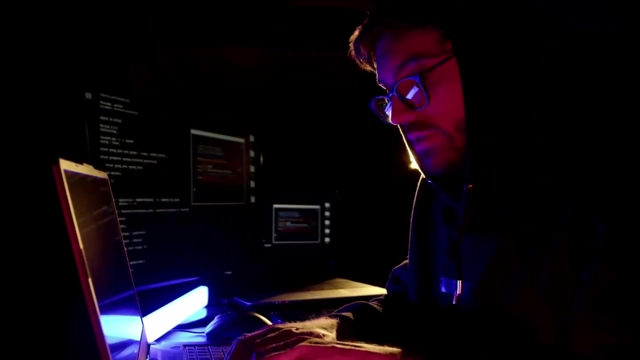 teach you everything you need to know. I love this method because you start learning the practical and marketable stuff immediately, but then you start preparing yourself for the long-term necessities. This keeps your motivation higher and it really just makes you marketable quicker. 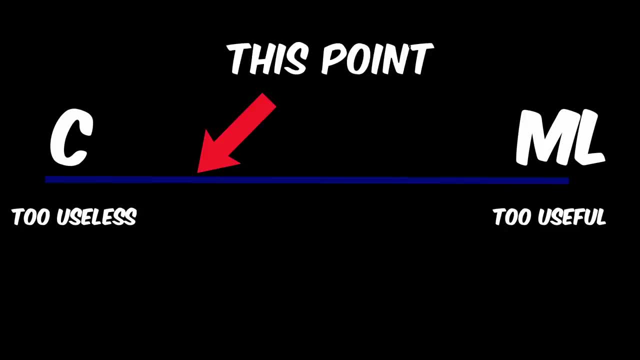 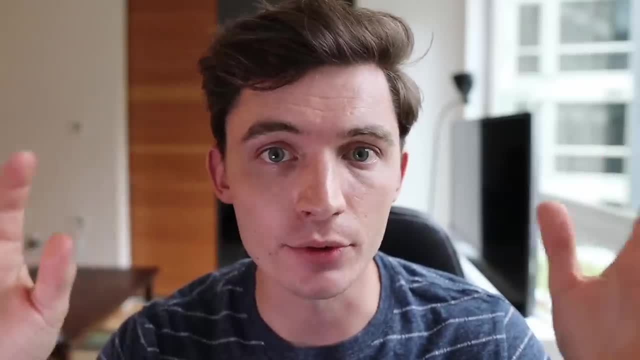 Now, what website should I build? Think back to useful, but not too useful. This doesn't need to be very complicated. In fact, it really shouldn't be complicated at all. There's going to be a lot of new ideas and concepts thrown at you If you try to build the next. 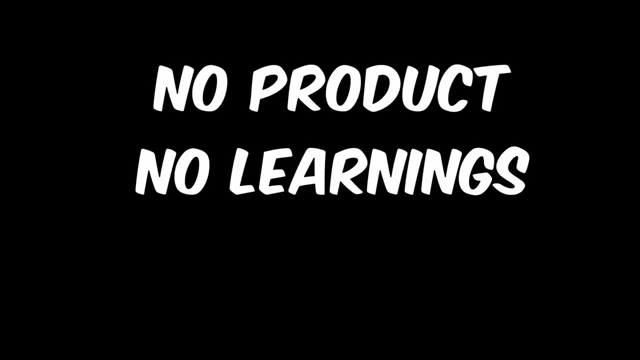 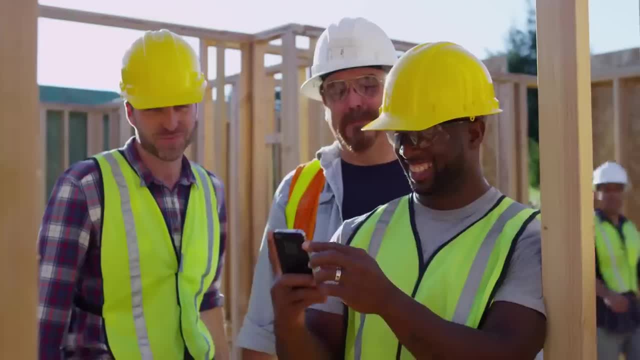 Tinder or the next Instagram, you're going to end up with no product, no learnings and no motivation. Now, before I give some concrete examples- and I will- let's talk about what makes a project good in an abstract sense. It's always best to create things that you actually find. 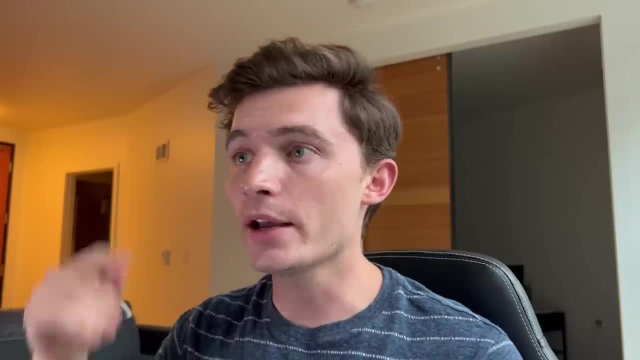 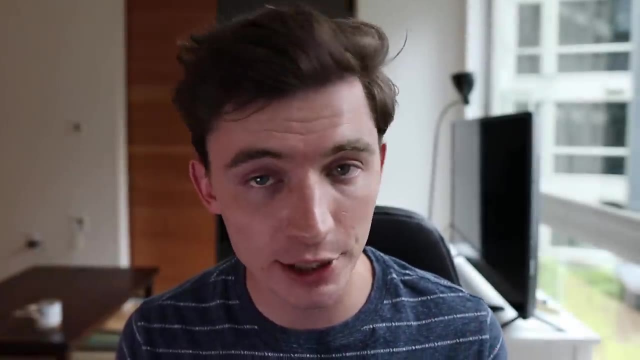 useful. I'll give you an example of one of my first side projects. So I created this thing called Spotify to YouTube MP3.. In university I had a trial of Spotify and when it ran out I was too cheap to buy Spotify. I didn't have any money, but I had 400 plus songs in my 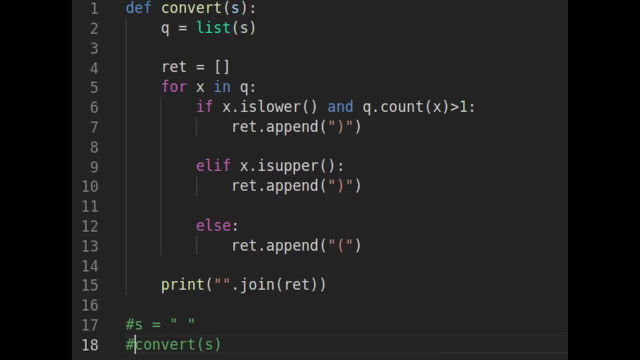 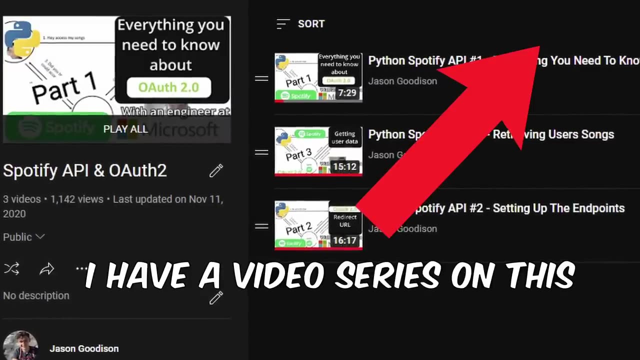 playlist. I didn't want to lose all that, So I created a Python program that uses the Spotify API to get those songs And then YouTube's API to download the MP3 version. Now I had all the same music, but for free. 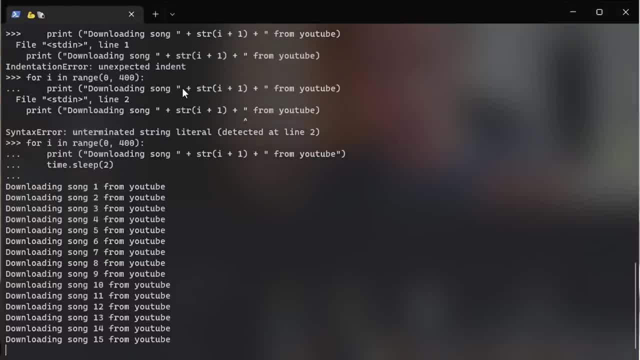 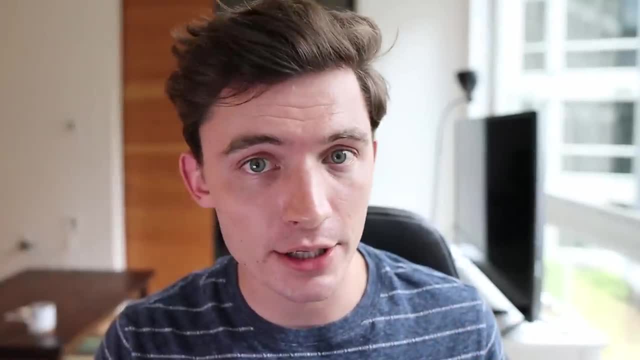 This project was one of the few that I actually finished And it's one of the few employers loved asking about Why? Well, one because it's unique, but two because I actually used it. I built it for myself. Other projects I would start, and then I would lose motivation. 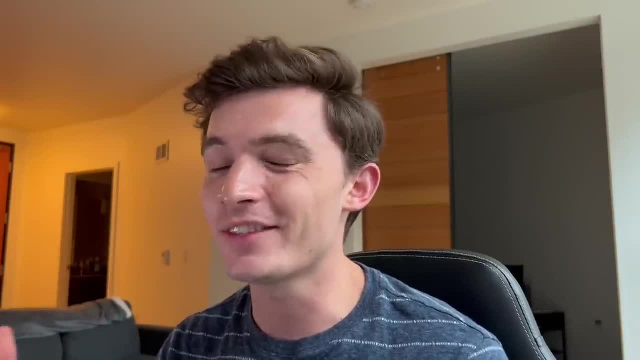 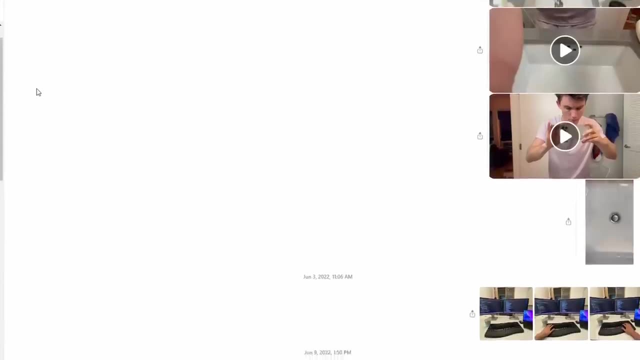 and I would never finish. Think a little about some problem that you have in your life that would be nice to know. Maybe it's just knowing when your favorite beer is on sale, or maybe it's an online clipboard so you don't have to keep messing around with it. Maybe it's just knowing when your favorite beer is on sale, or maybe it's an online clipboard so you don't have to keep. 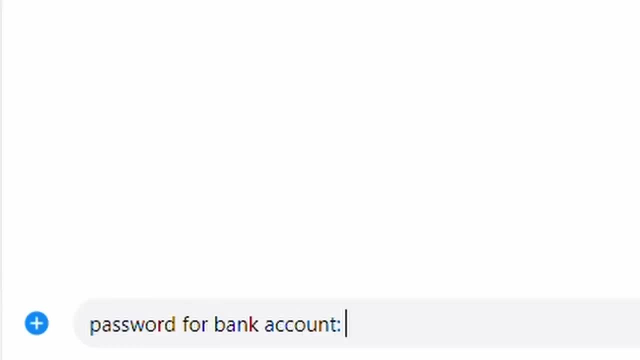 messaging yourself random shit on Facebook Messenger all the time. It doesn't have to be relevant for everyone. It really just has to be relevant for you. Now, if you don't have an idea yet, don't panic, I have a solution for that. You're allowed. 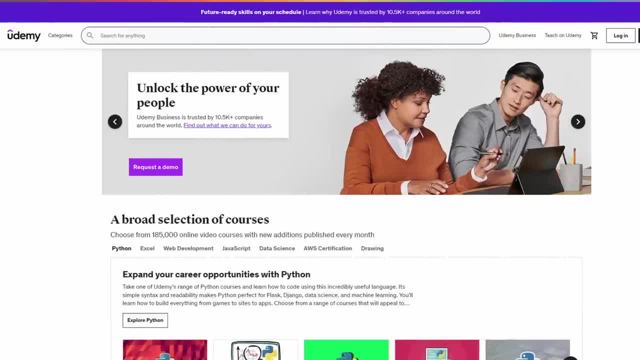 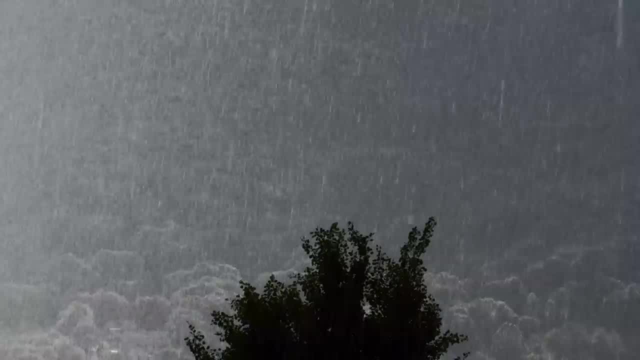 to follow a tutorial on YouTube or Udemy or any of those sites, but you're not allowed to build the same website as them. For example, if you're following a tutorial on how to build a weather website, instead try building something like a currency converter. That's a real example. 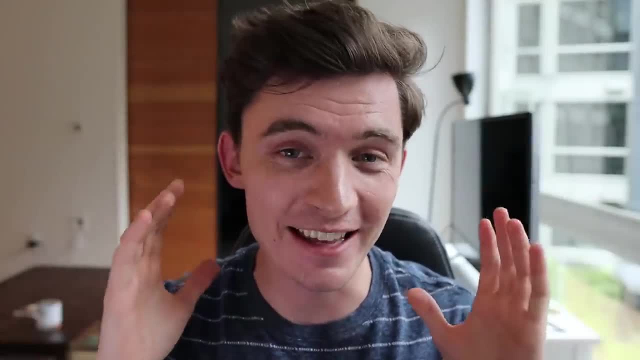 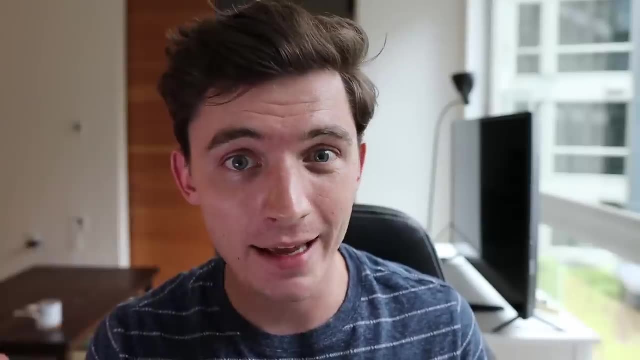 that I did. What's great about that is most of the code and the concepts are going to be the exact same. It restricts you from being able to copy and paste the solution. Therefore, you can follow the tutorial, but you can't copy it. 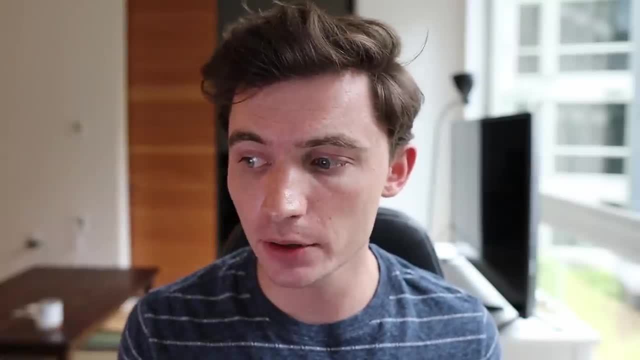 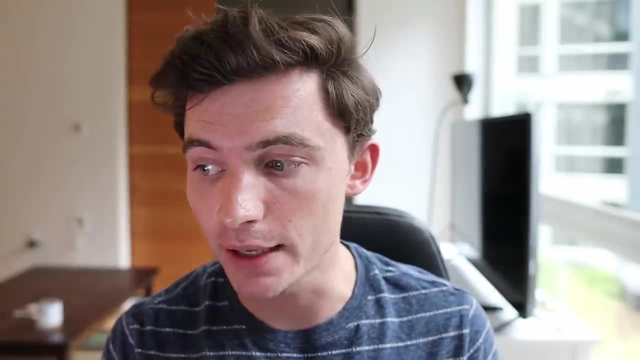 Now moving back to C, C++ for a second. The best and most popular languages and frameworks are always going to change. They're changing as we speak right now. Don't underestimate those fundamentals you've learned in C and C++ because, ultimately, if you know those well,